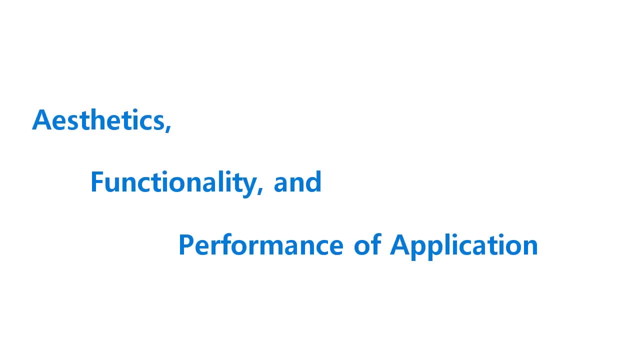 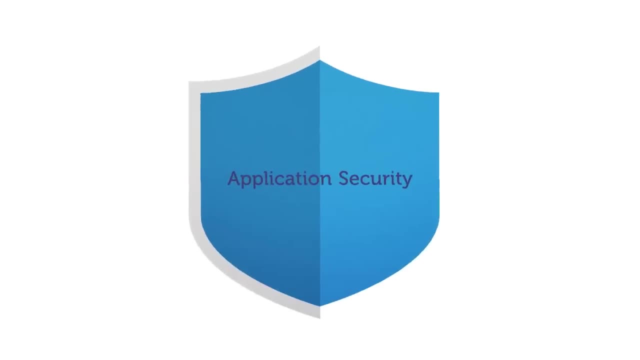 on the aesthetics, functionality and performance of their applications, and this inevitably means that they de-prioritize cybersecurity. In this fast-paced video, we want to show why application security is critical and how you can grasp key application concepts all in approximately 5 minutes. So hold on tight. 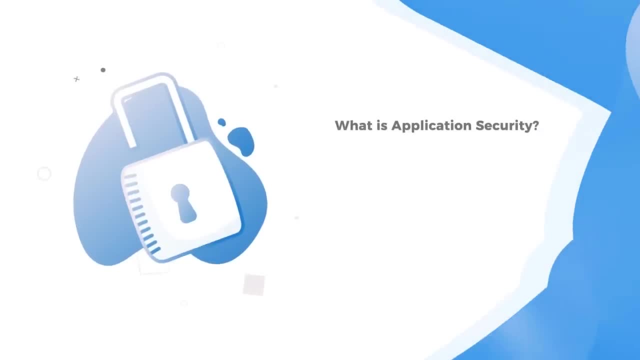 First let's get a clear picture. What is application security? Simply put, application security is an application security tool that can be used to implement applications in a way that is easy to understand. and easy to understand, Application security is the general practice of minimizing the vulnerabilities to your software. 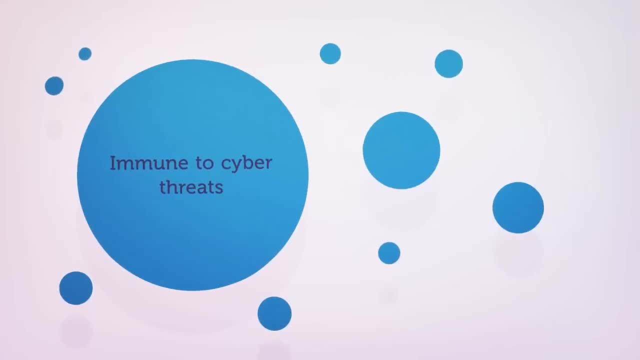 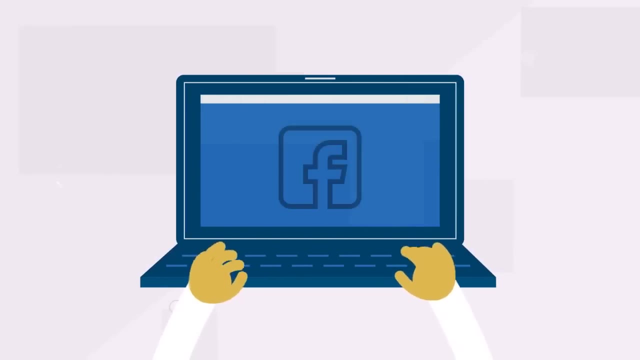 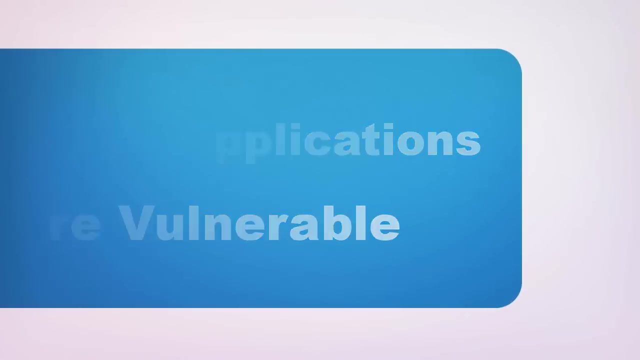 making it immune to a range of cyber threats. Every institution of economic and strategic importance today uses some software or application. Even the OS in your home PC is a type of software, and so is your Facebook account, a web-based application. Application security is important because 100% of applications today have some form of vulnerability. 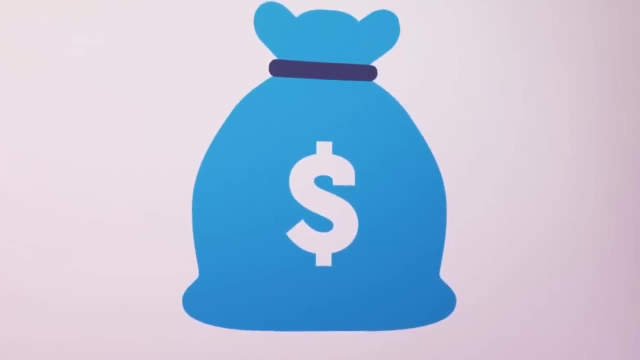 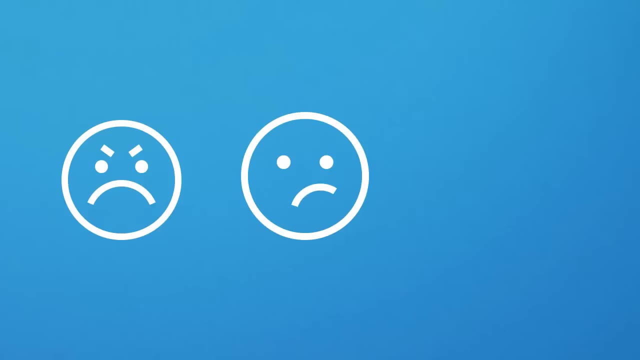 and there are trillions of dollars riding on these applications and their associated processes globally. Failure to adequately protect the applications of your organization may result in loss of trust, brand image and data, and expose you to huge penalties due to breach of various regulatory frameworks that your organization may be accustomed to. 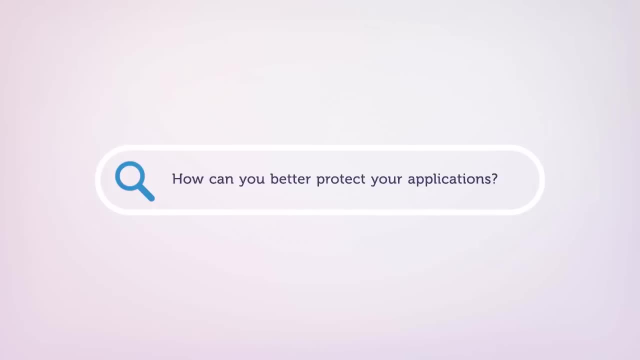 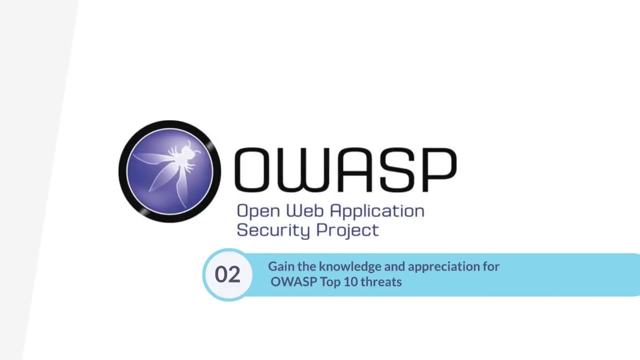 So the question is: how can you better protect your applications? The idea is simple. It is a 10-step approach. Step 1. Implement a secure SDLC framework for software development. Step 2. Gain the knowledge and appreciation for OWASP Top 10 Threats. 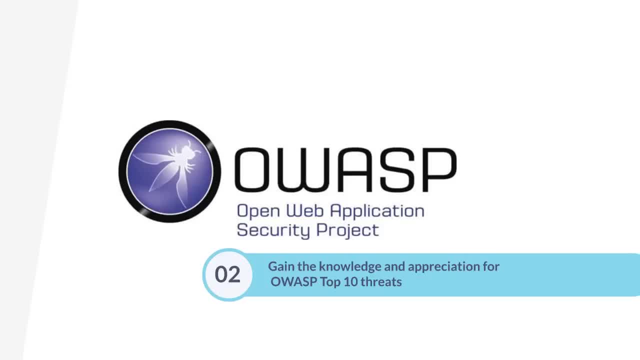 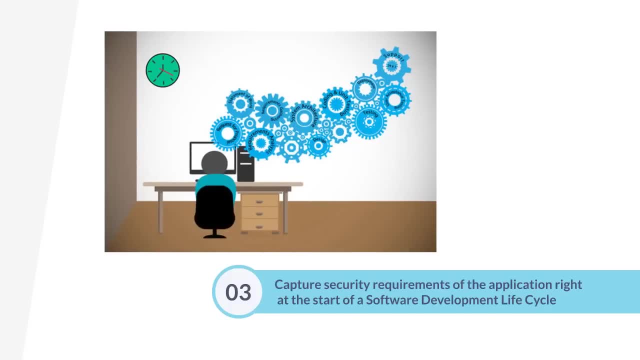 a globally recognized list of the top threats, which are updated annually. Step 3. Build the skills for threat modeling. Step 4. Capture security requirements of the application right at the start of a software development lifecycle. Step 5. Then you must define, maintain and enforce industry application security best practices. 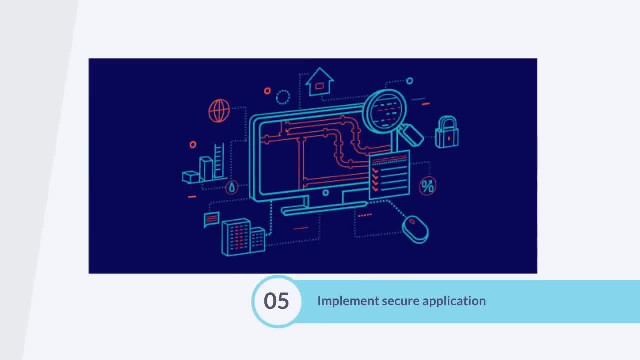 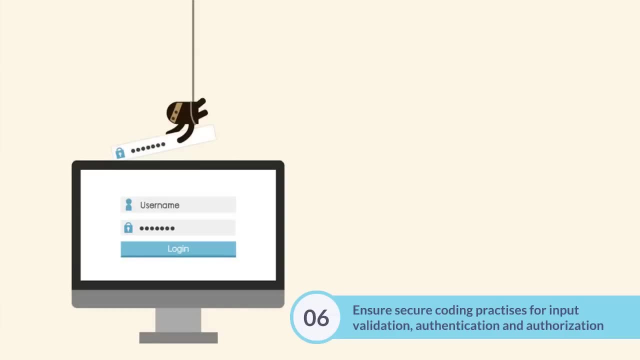 which evolve pretty quickly. Step 6. Implement secure application design and architecture. Step 7. Ensure secure coding practices for input validation, authentication and authorization. Step 8. To ensure well-rounded security of your application from the coding cycle itself. It's 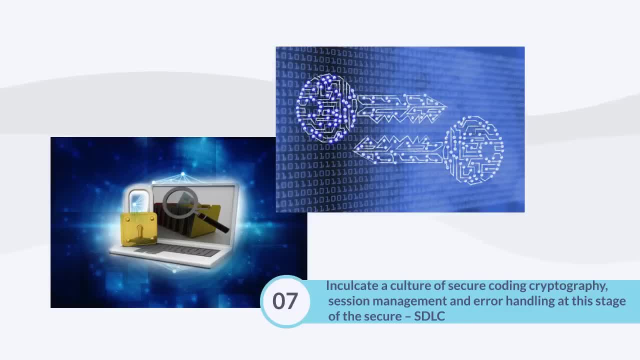 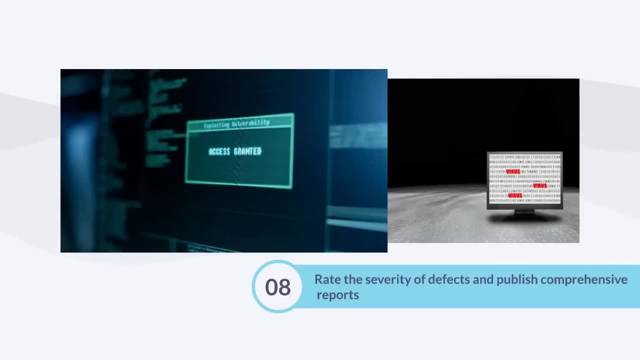 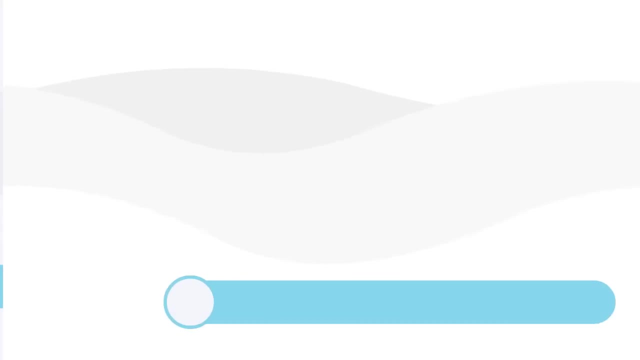 important to inculcate a culture of secure coding, cryptography, session management and error handling at this stage of the secure SDLC. Step 8. If some vulnerability still persists, rate the severity of defects and publish comprehensive reports detailing the associated risks and mitigations of the vulnerabilities. Step 9. Now it is time to scan your application. 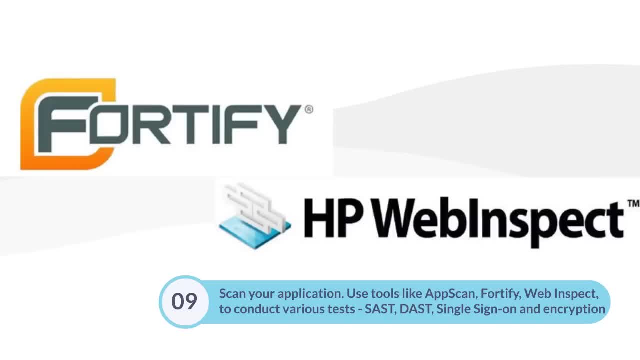 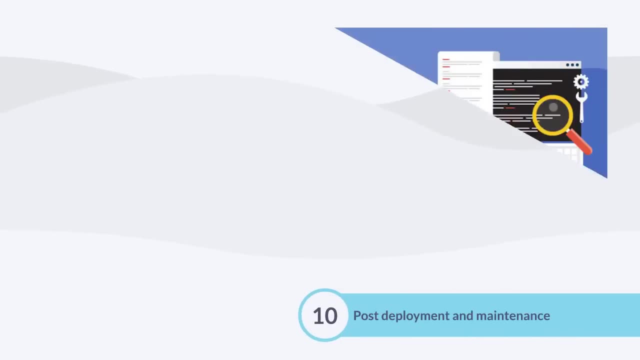 You can use any of the popular tools like AppScan, Fortify, WebInspect to conduct various tests, such as Static Application Security Testing, Dynamic Application Security Testing, Single Sign-On and Encryption Step 10.. Last but not the least, the process to implement application security must always follow the philosophy of creating 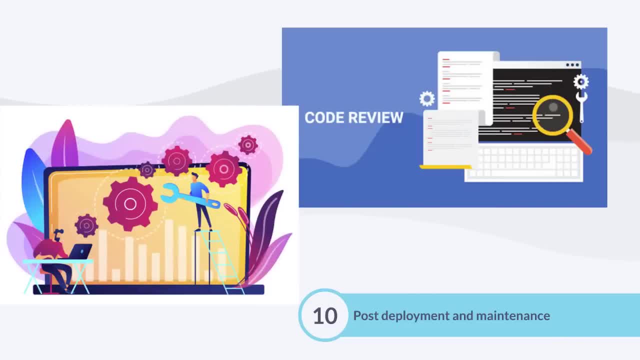 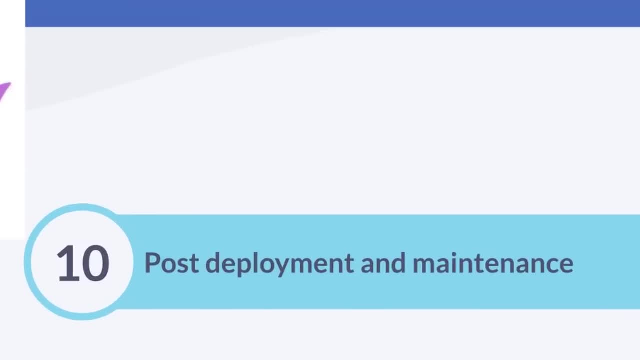 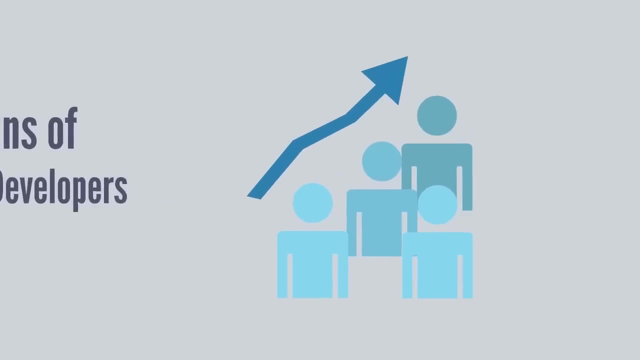 a software source code review process that is part of the development cycles. Perhaps the most admitted yet critical step in the SSDLC framework is the post-deployment and maintenance phase that ensures security at various levels. With millions of software developers employed across the world, development companies have just too many professionals to 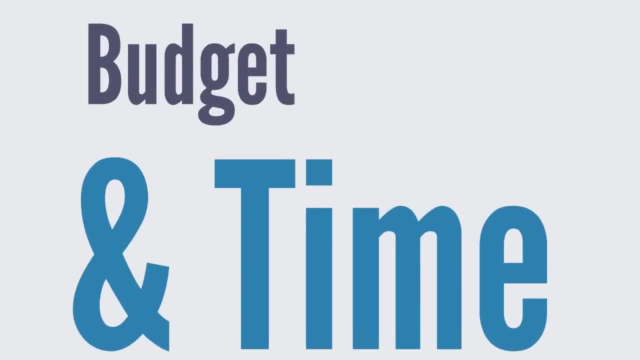 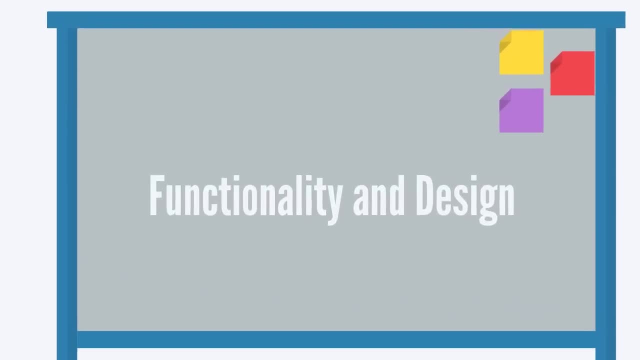 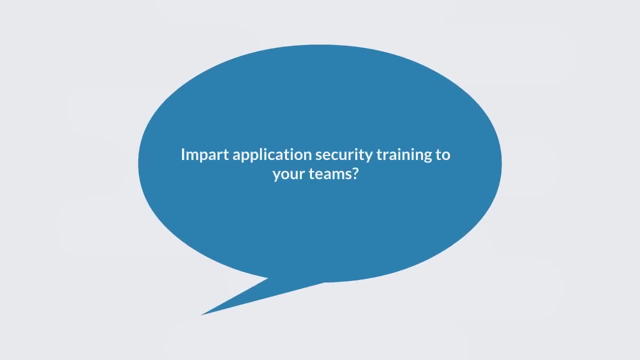 train. Budget and time constraints are factors that make matters worse. The vast majority of undergraduate programs in computer science do not focus on application security. Rather, the focus is almost entirely on the functionality and design of the applications. So how can you impart application security training to your teams? 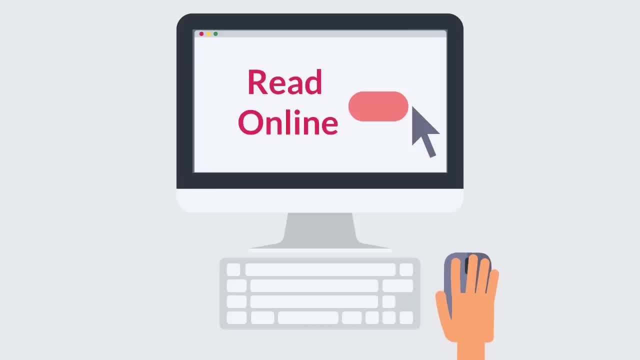 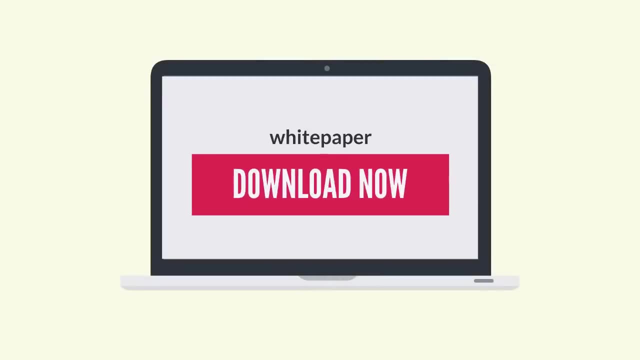 Well, of course, you can do it in the old-fashioned way. You can read many books online on the topics shared earlier, then stay up to date with the recent developments on these by reading through the many white papers published in this field. Do not stop there. 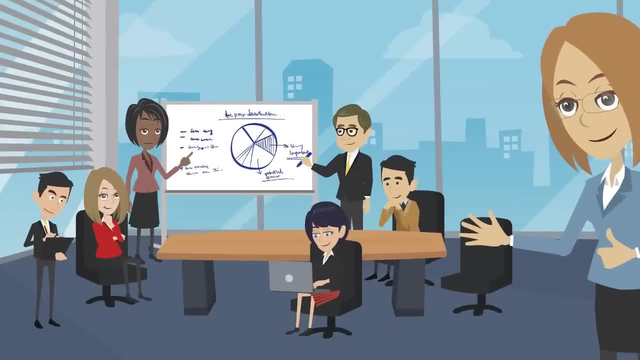 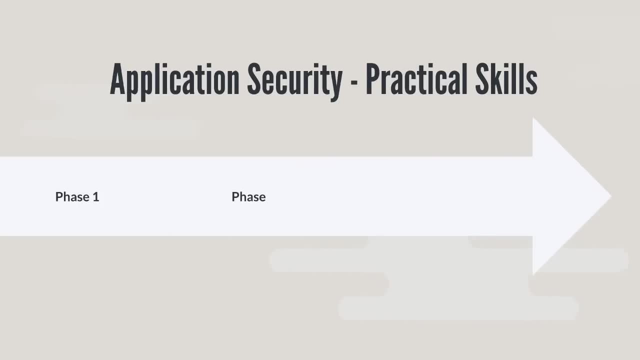 You must make it a part of your routine to speak to consultants and interview them to get a leadership perspective. However, while the steps above may be effective to train your application security workforce, practical skills will still need to be imparted- An effective way to do that. 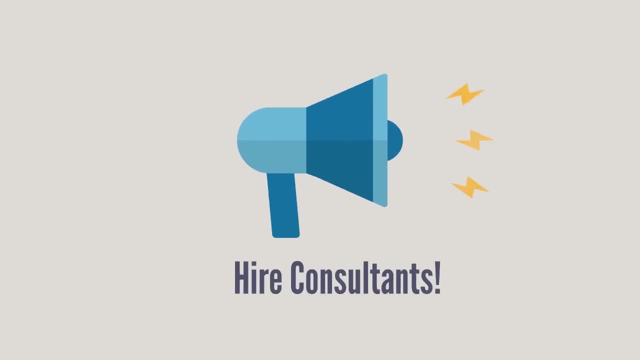 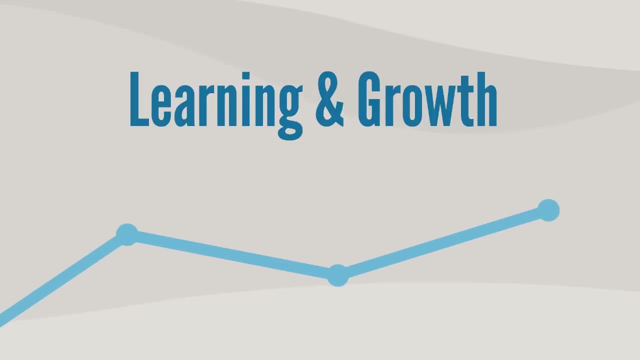 could be to hire consultants to train and test your products. This can be expensive, but worth it. Then make sure you are able to manage the learning and growth of your teams in application security, while ensuring that they do their job, roles assigned and deal with attrition at the same time. 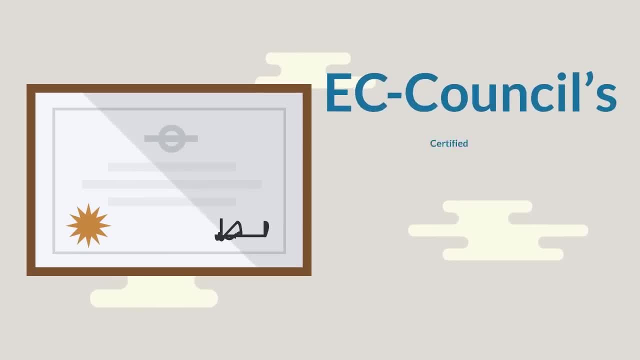 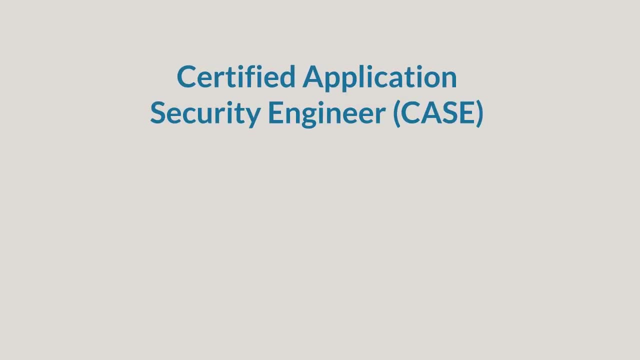 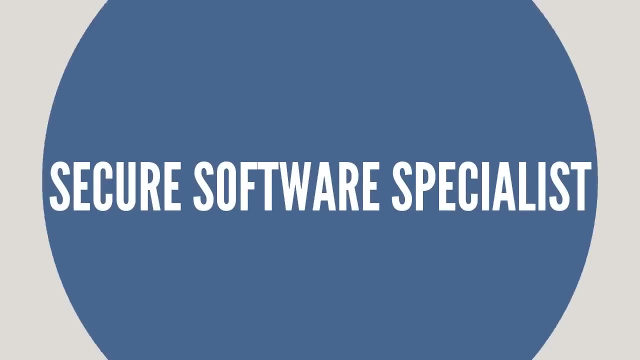 There is an easy way as well: Introducing EC-Council Certified Application Security Engineer Program. The Certified Application Security Engineer Program, or CASE for short, available for both Java and NET, can make your team of software developers secure software specialists in just three days of training. 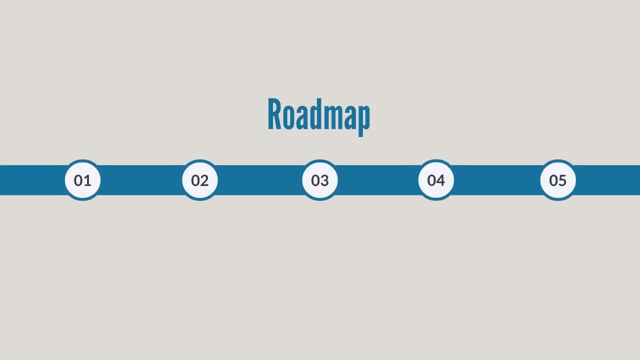 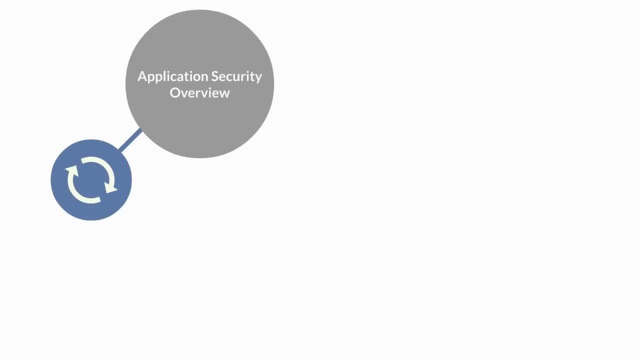 Covering the entire spectrum of a secure software development lifecycle and beyond. CASE spreads its training over ten modules, beginning with an overview to application security and attacks. You will begin by gaining an understanding of the most common application level attacks, including OWASP top-then threats. Then you would undergo a surgically segregated